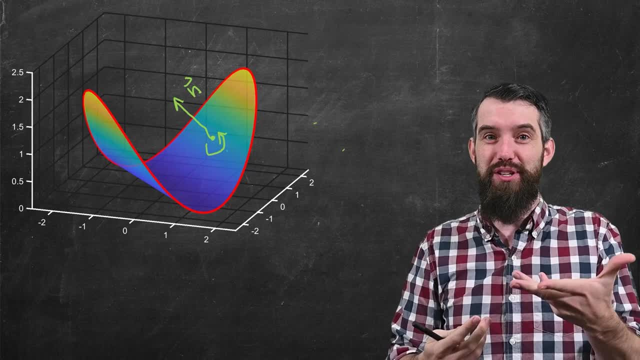 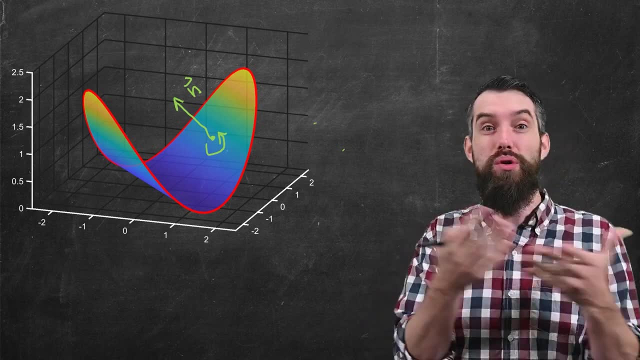 for example, my particle is not free to go anywhere. they have to go on the surface, but they're still influenced by the vector field. then they may rotate counterclockwise or clockwise faster or slower in this little region around the point that has normal vector, this n, And indeed 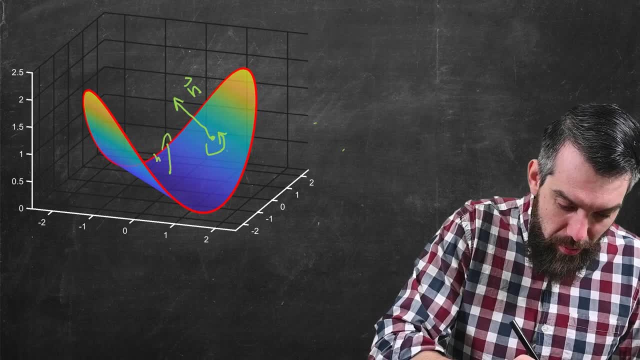 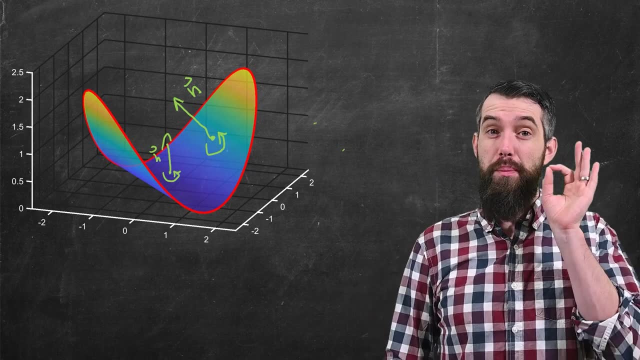 I can go to any spot here, anywhere on the inside, and I'm going to have a normal and I'm going to have a little bit of swirling in the surface that's influenced by that vector. So I'm going to have a normal vector field. Perhaps what is most important is if I go to a spot that is right on. 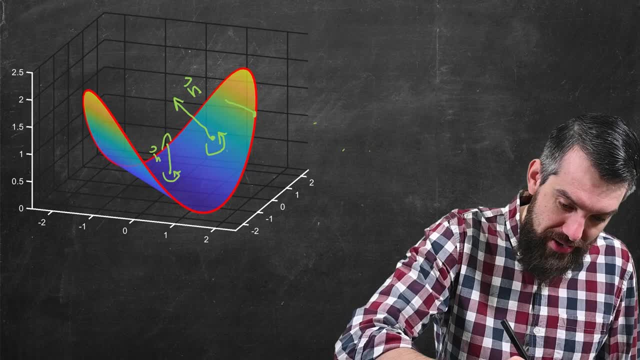 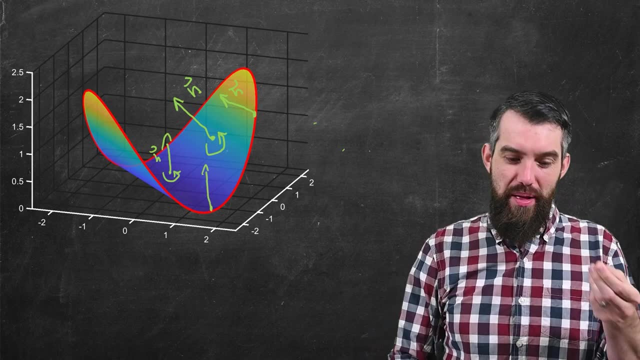 the boundary like that one. So now it looks like the normal vector might go something along the lines of this, Or perhaps down here and it would go more vertically, But at either spot likewise there would be a little bit of swirling going around, And here's the key point Again. 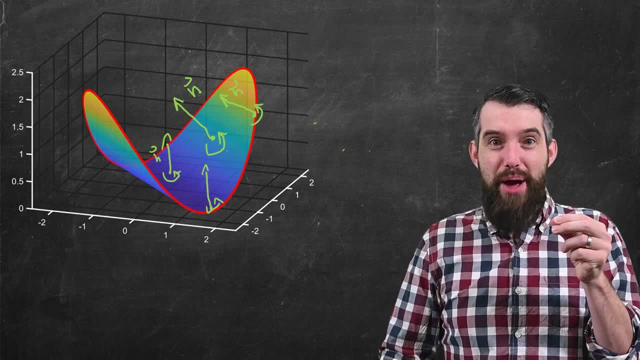 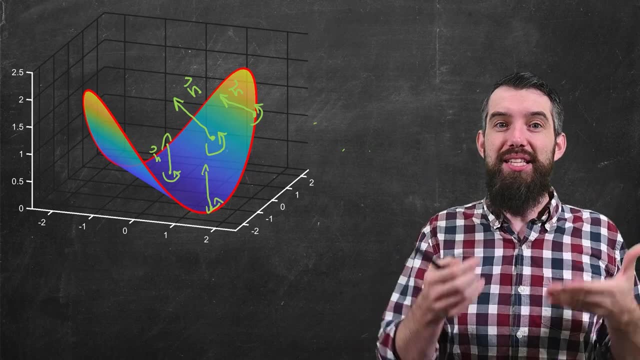 imagining I've got some sort of velocity field here. If I'm on the boundary and I want to ask the question: what is the circulation around the boundary? Well, the key point is that the tendency to circulate along that boundary is going to be influenced by that curling at each. 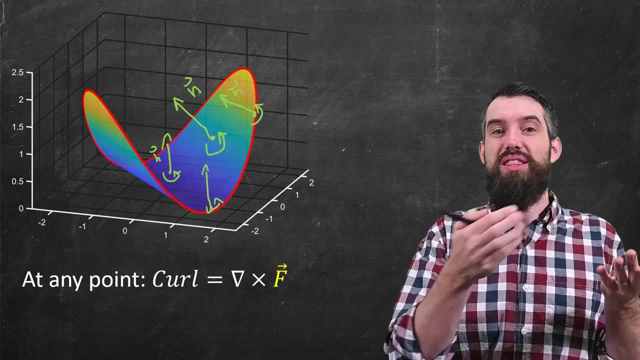 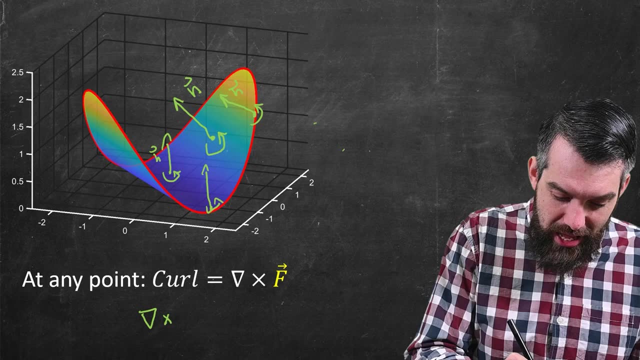 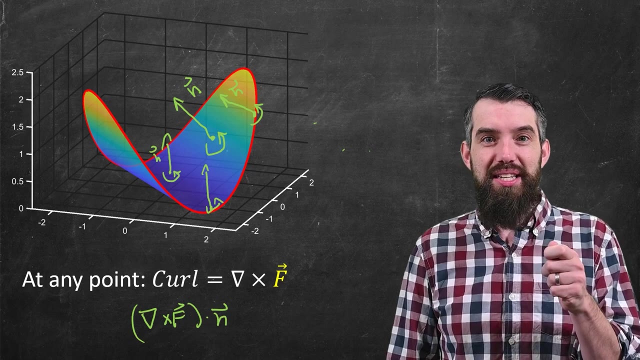 point along the boundary. So the general formula, as we've seen, is that the curling point is given by del cross f. But then if I form del cross f and dot it with the normal vector, at that point that gives me the tendency to- how should I put it? curl within the surface. That is the curl sort. 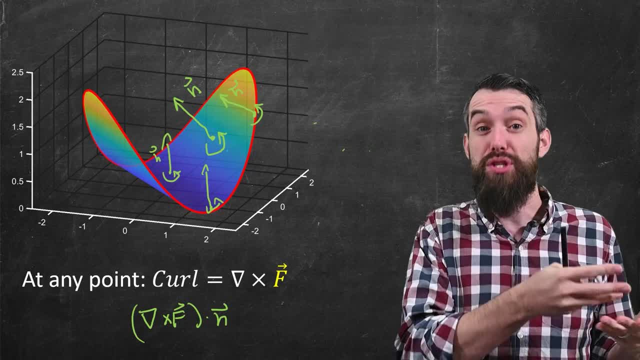 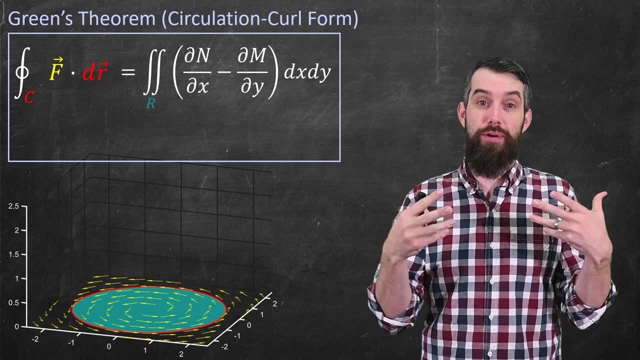 of is subject to the constraint that we must remain on the surface Before we get to Stokes' theorem. I want to go back a little bit and talk about Green's theorem, because in many ways Stokes' theorem is a generalization of Green's theorem. So the picture for Green's theorem is more or less. 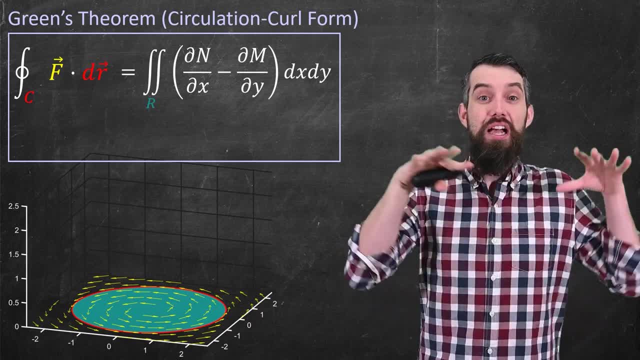 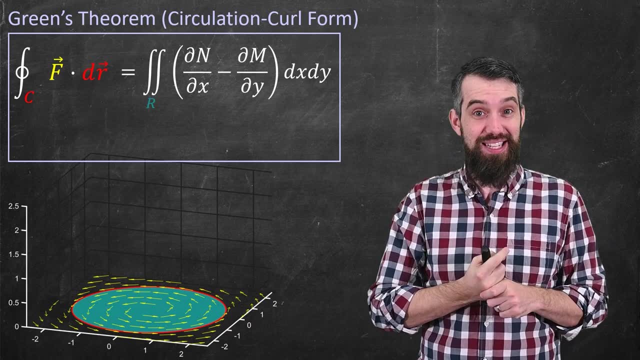 the same scenario. It's just everything exists down on the plane. It's a two-dimensional version of it And because I'm going to upgrade to three dimensions, I just drew the two dimensions in the plane, but I included the third axis because we want to add some stuff there in a little bit. 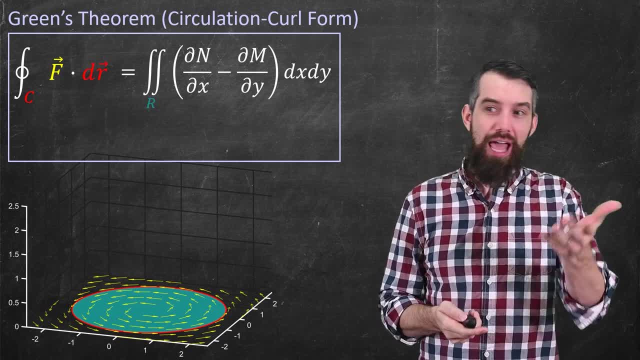 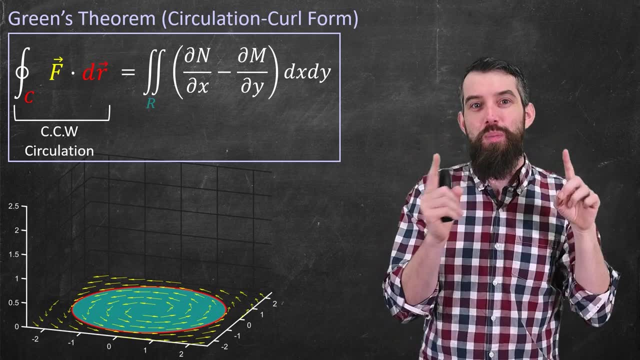 And so when I look at this theorem, what it's really saying is: on the left, we have that counterclockwise circulation, as we were talking about the tendency to circulate around the boundary, And what was remarkable about Green's theorem was that this was just equal to a double integral over the entire region, including all of 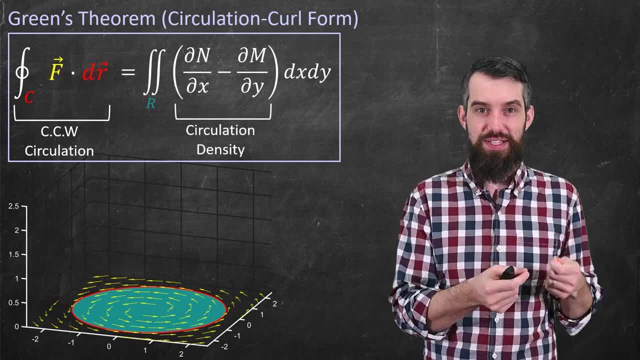 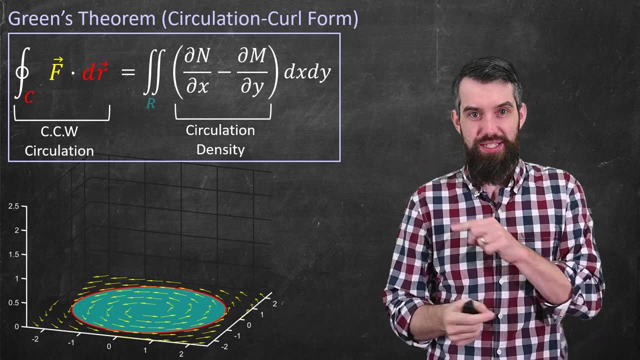 that inside of something that we call the circulation density. What I'm going to do, that's new about Green's theorem, is just add a little bit new terminology. So you know how about the circulation density? this difference of these partials? Well, we saw in the previous video. 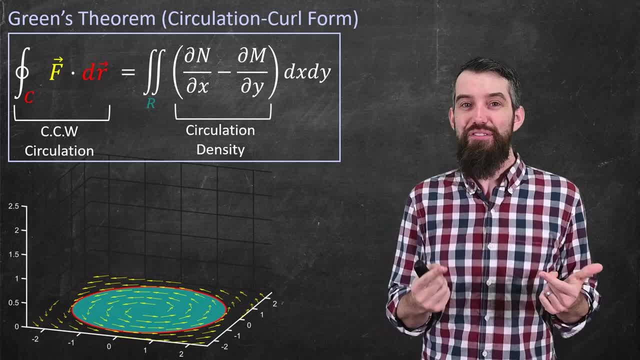 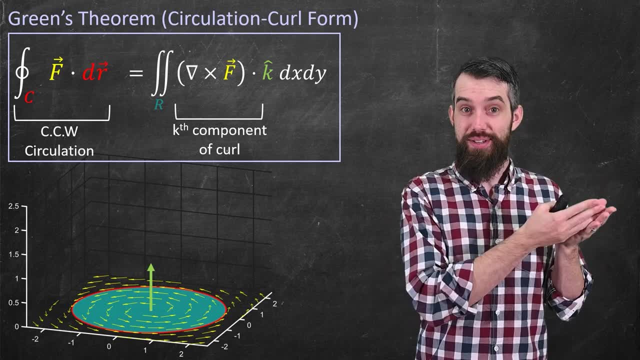 the curl of a circle, And so what we're going to do is we're going to add a little bit of vector field, And indeed what I have here is just the kth component of curl, And so I'm going to replace that, I'm going to rewrite this as the curl, which was this: del cross f dotted with k hat. 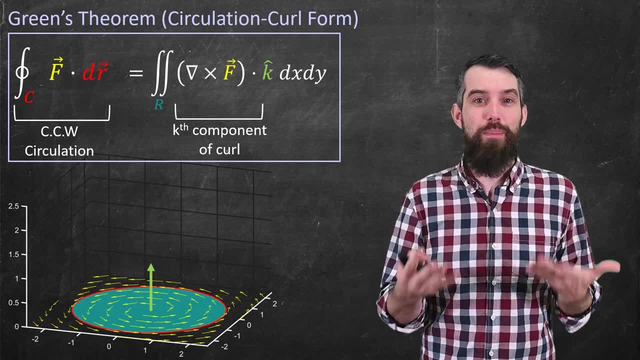 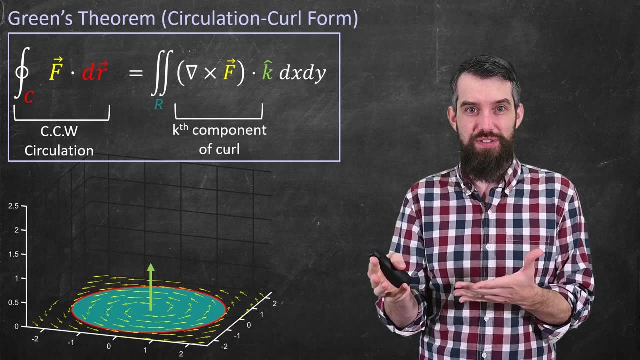 where k hat in my picture is sticking straight up out of the xy plane. So we have this upgrade on Green's theorem, which really is just a terminology or a symbolic shift. We had this thing defined to be the curl, and I just recognized it as part of what was in Green's theorem, And so I've just 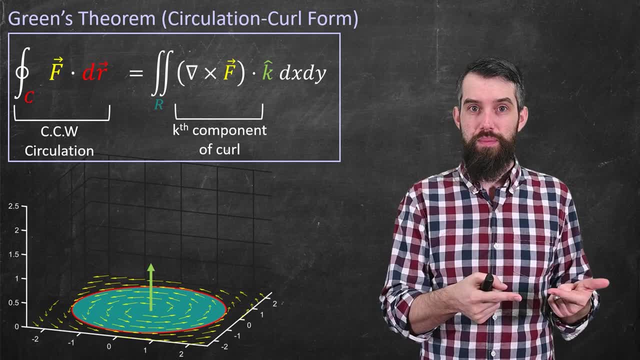 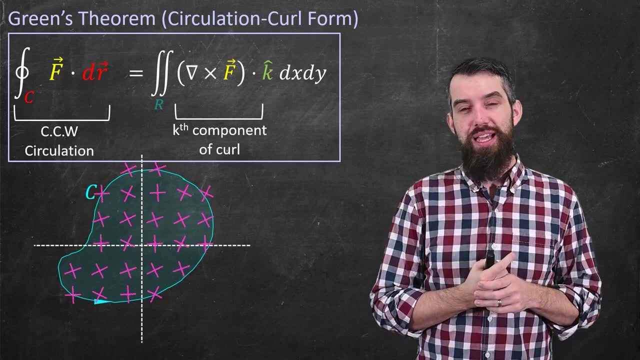 added the curl here, the del cross f, and then dotted with k hat, Another way to visualize what's going on a little bit better here. so I'll drop the three-dimensional perspective and just look at this. two-dimensional is all of these little spinners that I've drawn here sort of regularly. 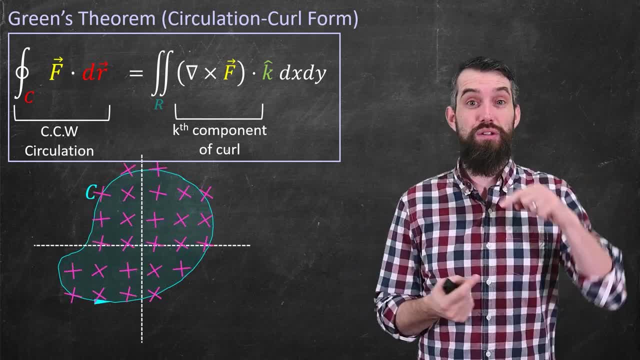 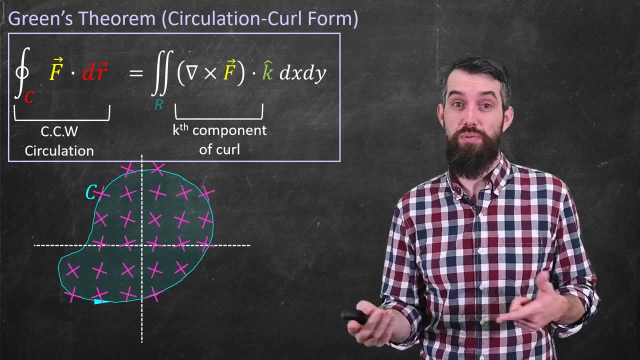 spaced out, give the tendency for this vector field to curl around at that particular point, at least curling in the xy plane. It depends on what the vector field is to know, whether they're going to curl counterclockwise or clockwise, fast or slow, But the argument is going to be. 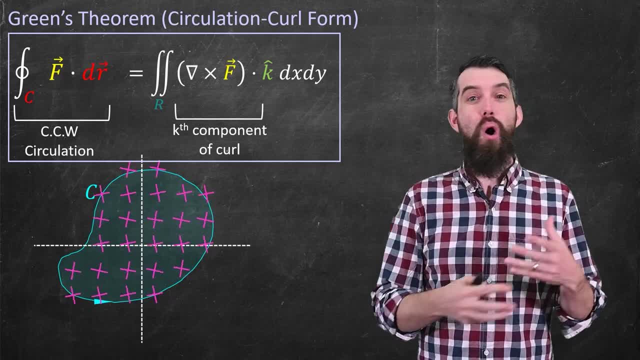 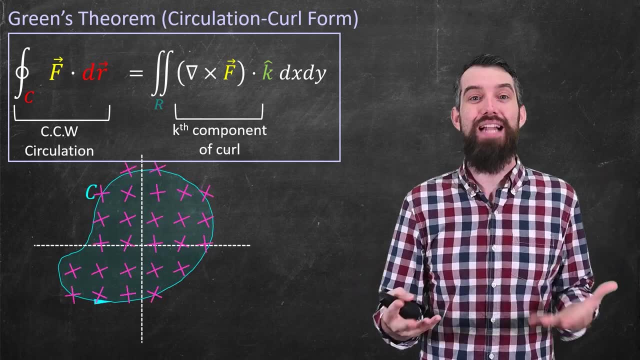 that in the interior, everything is just going to cancel out and all that's left of all of this curling around is going to be the proportion. when you add it all up together, that's around the boundary, and the boundary adds up to the circulation. The argument for why it cancels is: 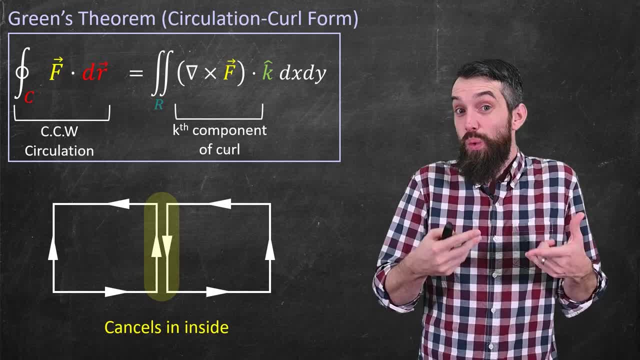 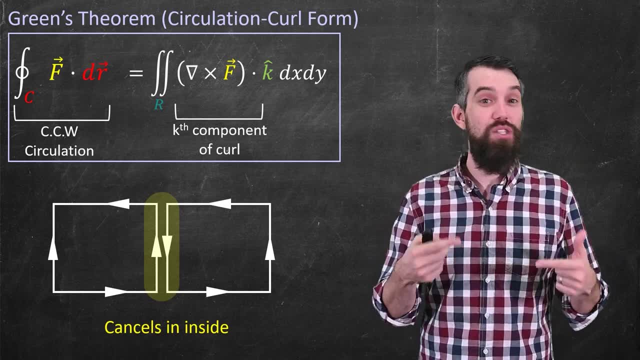 that if I have two adjacent little paths, then where they meet in one path it's the flow going up, and then in the adjacent path it's the flow going right back down again, And so it exactly cancels in all of these interior portions. All right, so now let's go to Stokes'. 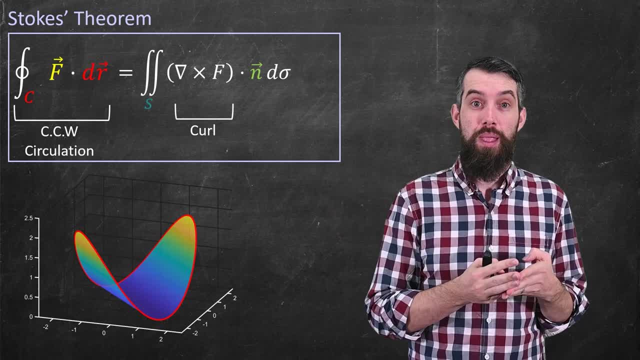 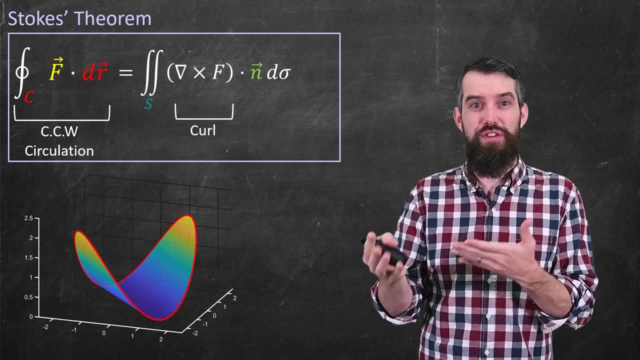 theorem. The first immediate difference is actually in my visualization. My surface is now a three-dimensional surface versus a two-dimensional surface. My vector field is a three-dimensional vector field, not a two-dimensional one. The left-hand side of Stokes' theorem is exactly. 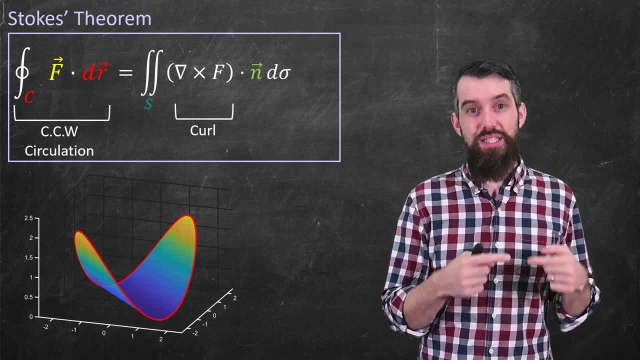 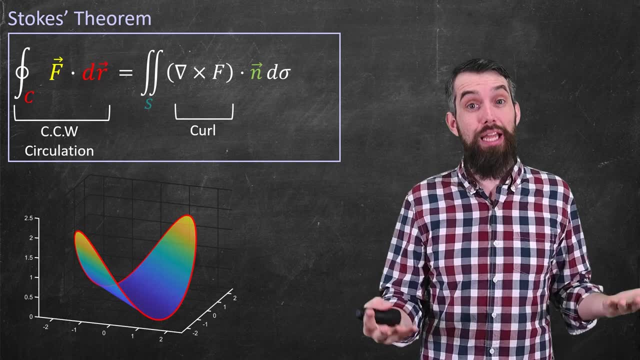 the same. It's the circulation around that boundary curve. Yes, it's the circulation around a curve that lives in three dimensions as opposed to two dimensions, the way it was in Green's theorem. but it's the circulation around some curve. And then, on the right-hand side, a couple 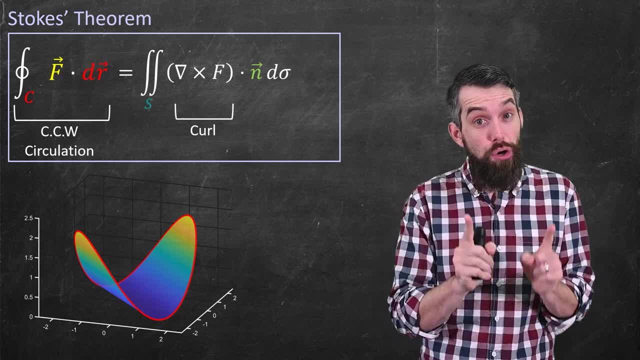 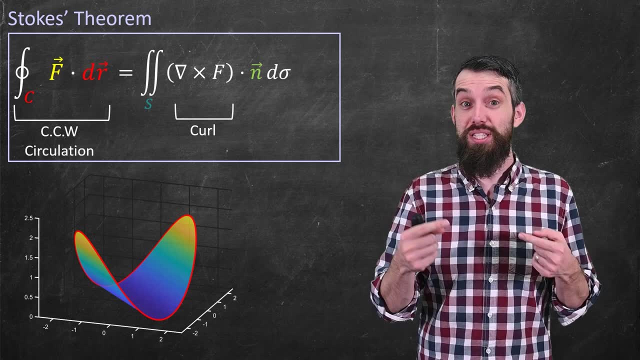 of things changed. First of all, instead of being the curl dotted with k-hat, it's the curl dotted with the normal vector, And that's because as you move to different places on your surface, your normal vectors are different things. It's not just k-hat everywhere the way it was for. 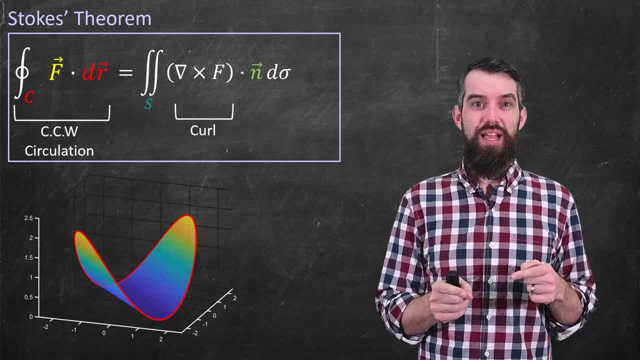 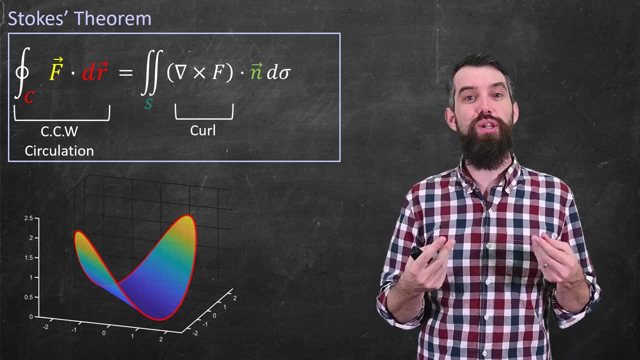 Green's theorem. And the second thing that's changed is that instead of in Green's theorem, where I was taking a little area down in the xy-plane, this is now a surface integral. It's an integral d-sigma as opposed to dxdy or dA as we would have had before. But the sort of intuitive argument for this is that it's a surface integral. It's an integral d-sigma as opposed to dxdy or dA as we would have had before. But the sort of intuitive argument for this is that it's a surface integral, It's an integral d-sigma as opposed to dxdy or dA as we would have had before. 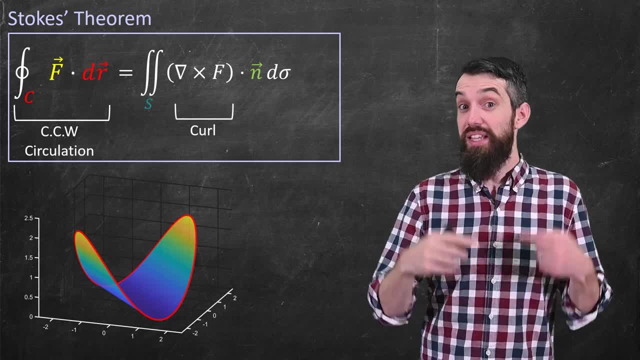 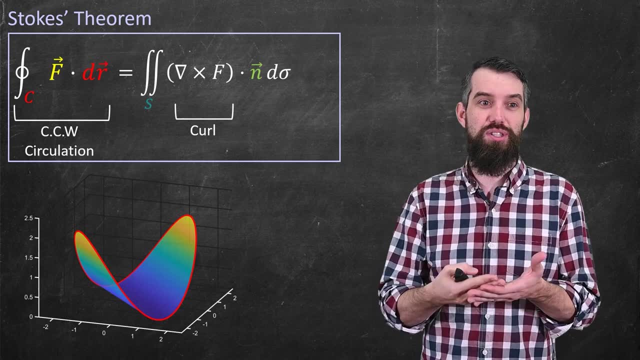 But the sort of intuitive argument for why this is true is almost exactly the same. At any point in the interior of this surface I have some curling that is measured by the curl of f dotted with n. So the curl, that sort of, lives inside of the surface, if you will. 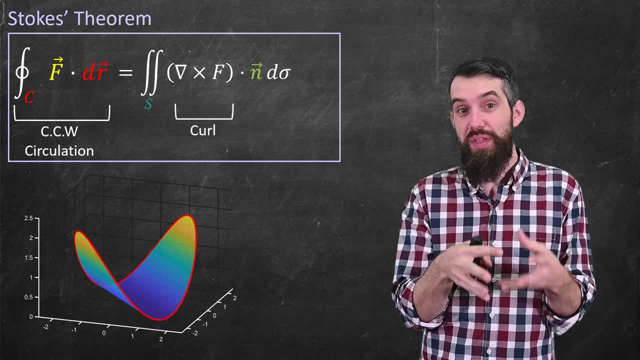 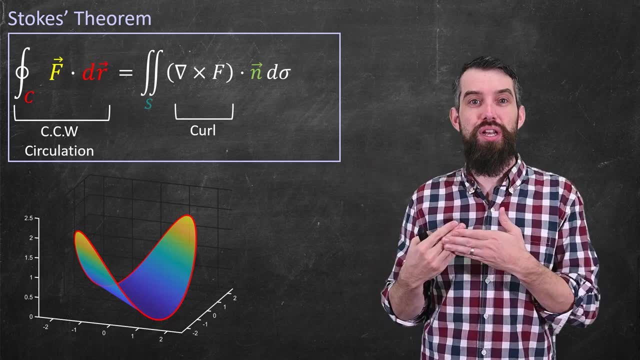 And then, if you add up all of the tendencies to curl everything along the inside cancels and just leaves with the curling along the boundary, And the curling around the boundary is what causes the circulation around this boundary curve. I do want to put up the conditions for Stokes. 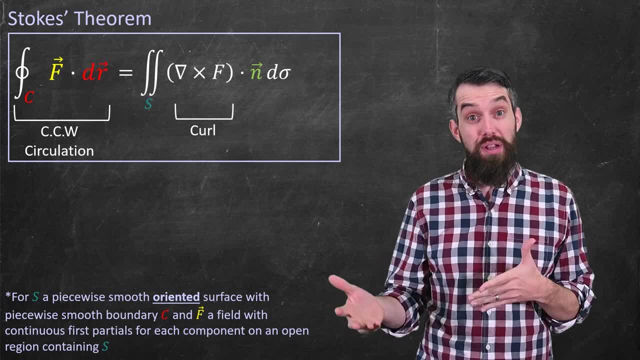 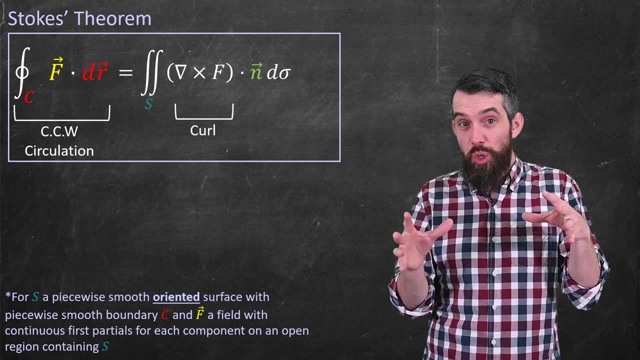 is theorem. the field has to be nice- in this case continuous, first partial derivatives of its modules- And the surface's ha s to be nice. It needs to be a smooth surface, or at least piecewise smooth, Like, for example, a cube has those boundary edges and corners and we still call the cube 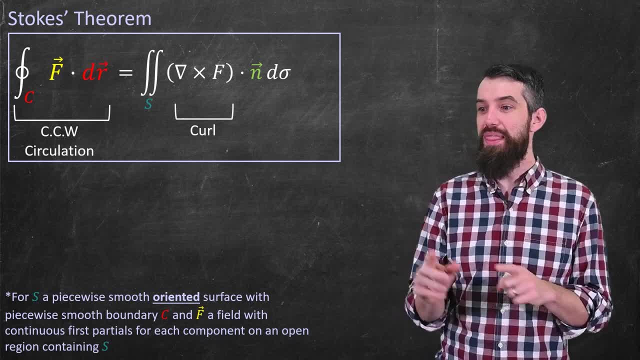 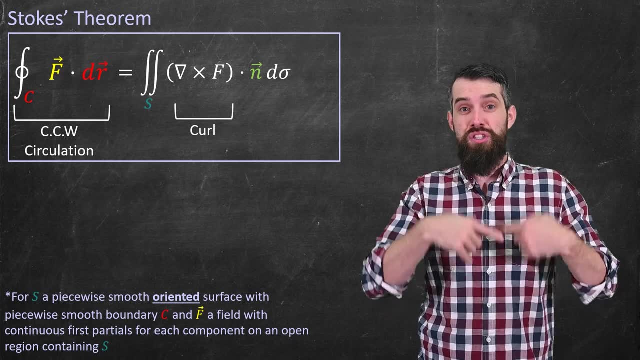 piecewise smooth. The real one that I want to focus in here, though, is the demand that it's an oriented surface We'd seen previously. an oriented surface meant the surface only had two different sides, and you could choose a consistent or a continuous choice of normals. 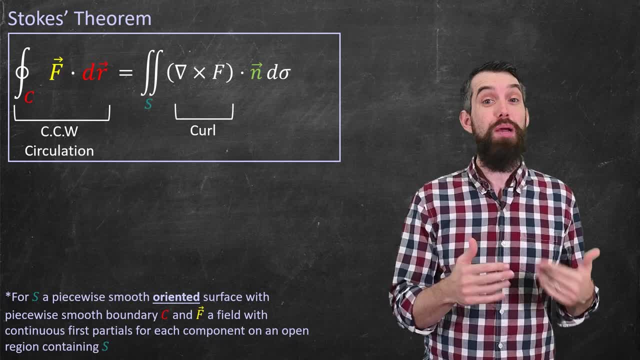 So if a plane was a plane then I still couldn't have if I chose a openuela and all its part sofit wrong. So I'm just Tory. people seem to have had certain normal results and let's assume that the Aquí normals to be able to compute the right-hand side of Stokes' theorem And so Stokes' theorem really.